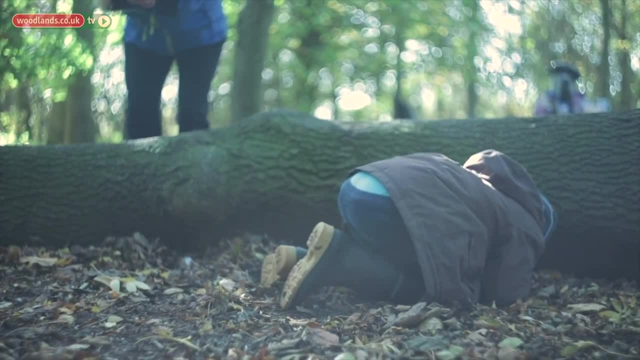 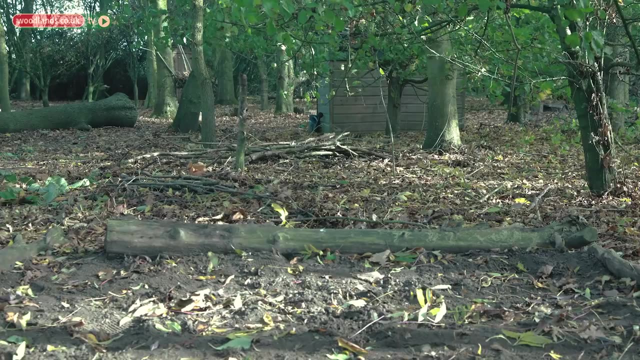 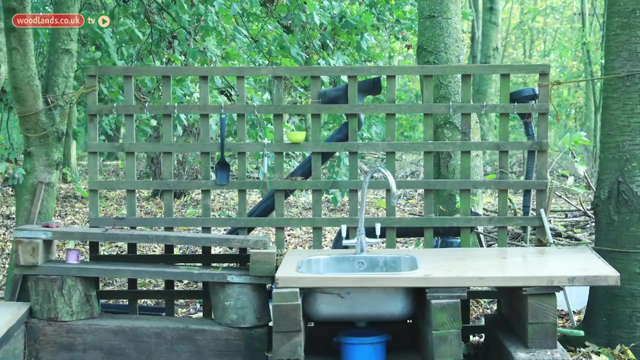 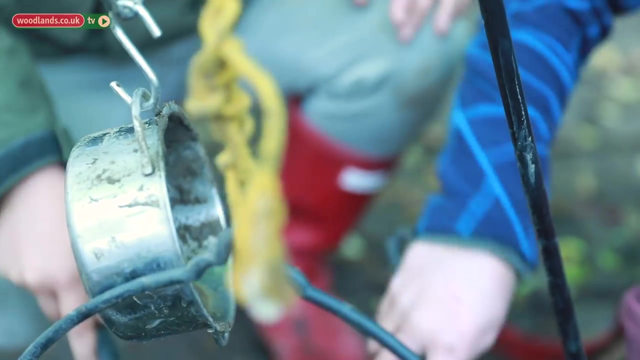 in the woodland to being in the woodland. One, two, three. where are you? One, two, three, where are we? Where are we all at? So I always have a digging area and I have a little mud kitchen area. We've been making apple mud pies, muds, water, dirty water, apples. 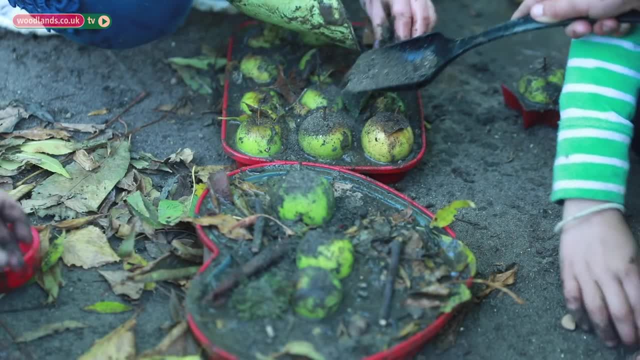 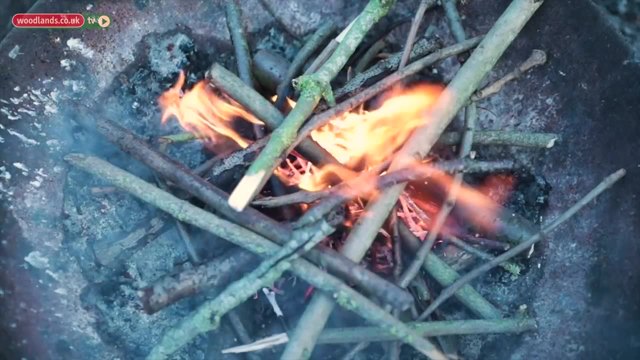 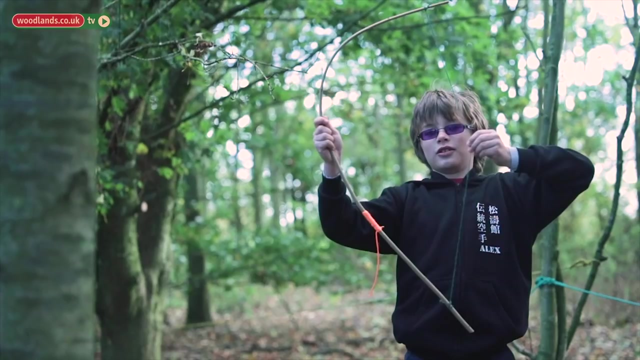 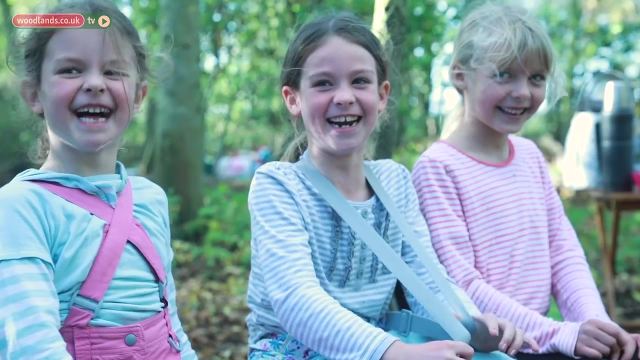 twigs, leaves, anything we can find on the ground. really, In the afternoon we usually have a fire and we do some cooking or something like that. The fact that the natural environment provides so many resources but also it doesn't provide everything, so they have to kind of think creatively. As the day goes on, they go off. 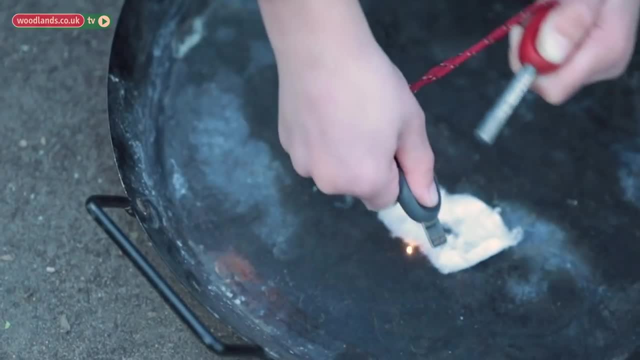 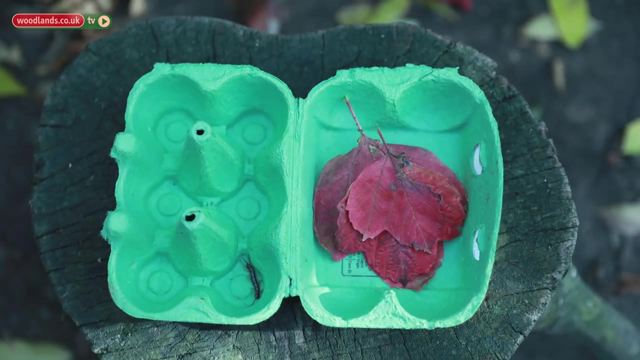 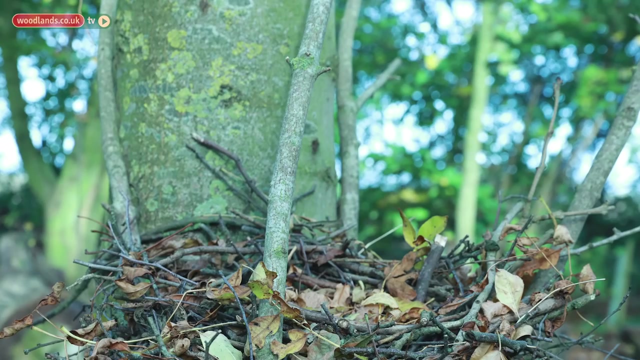 they make friendships and they find their own play and their own games, which is great. great to see. Egg Box Challenge, A mini beast, red leaf, shiny berry, something prickly soft, feather, something beautiful. Oh, one little wood flew out today and I got it. 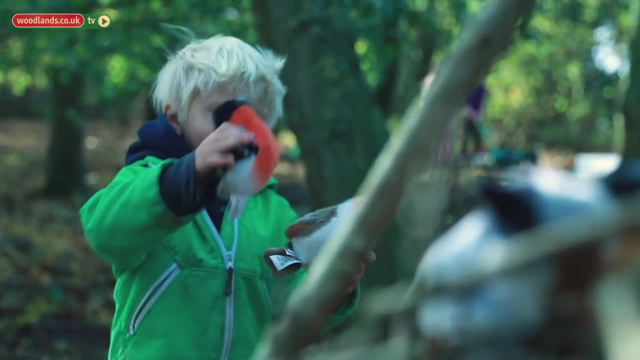 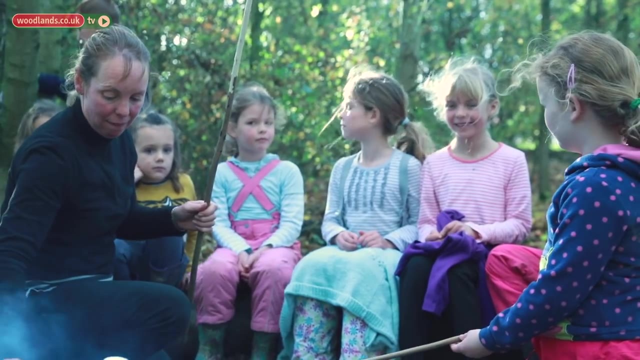 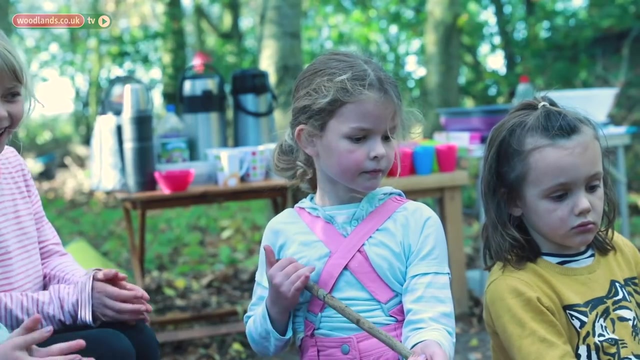 Oh, one little wood flew out today and I got it. Oh, one little wood flew out today and I got it. It's two days, Not a little weapon. What the parents get is a day or two days when the children don't ask at all to have. 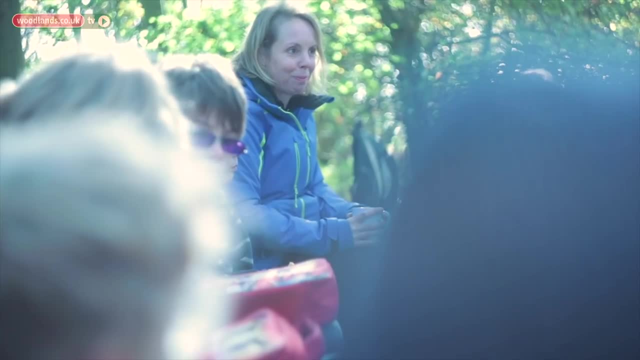 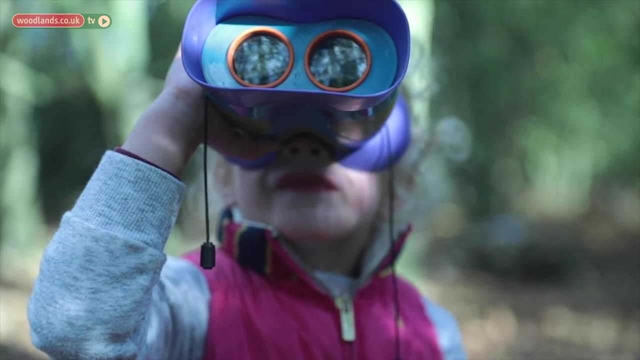 a screen. They just don't need it because they're just busy all day. And it's lovely, to be honest, because particularly with the little ones they always they notice maybe a toadstool that's appeared that wasn't there before. 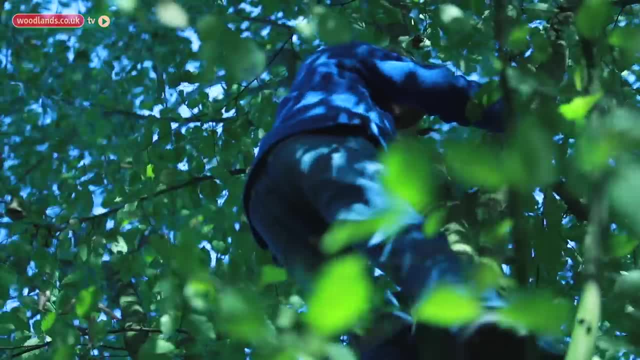 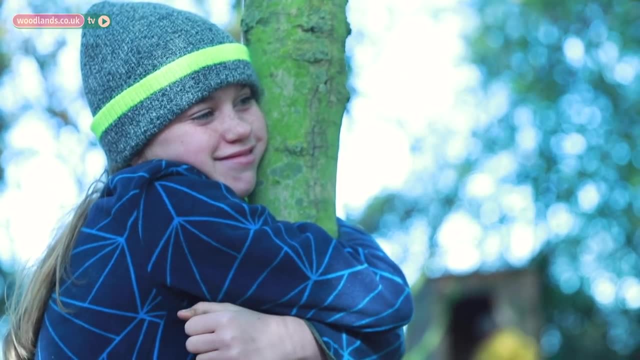 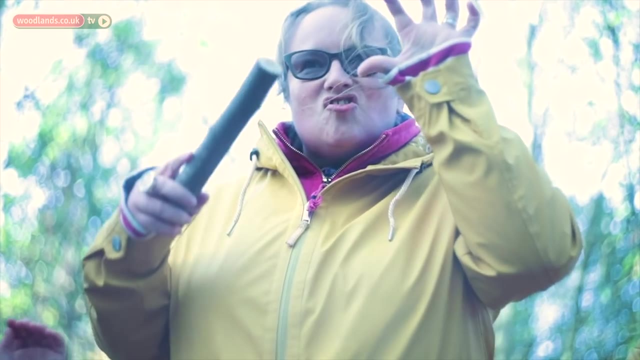 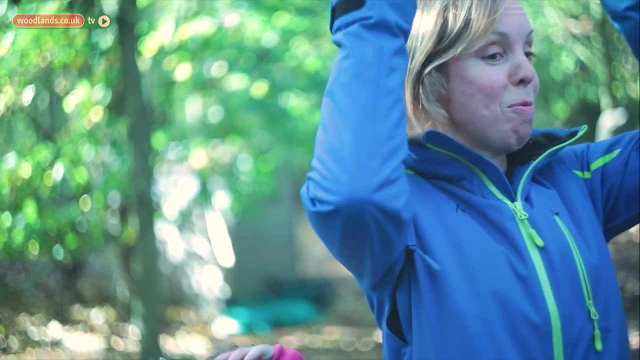 There are three things based on earth education principles. so it's about looking after yourself, looking after each other and looking after the woodland. and we try and leave the woodland. as we found it, Forest School is very much not focused on an end product.